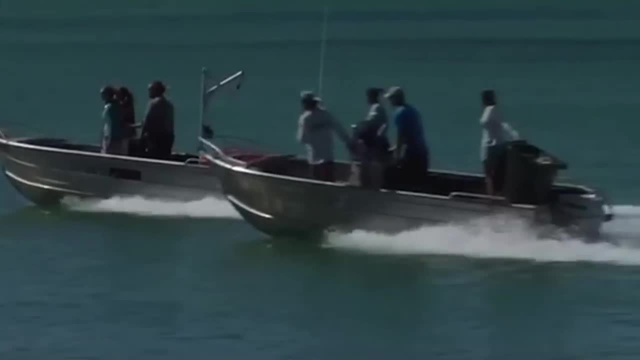 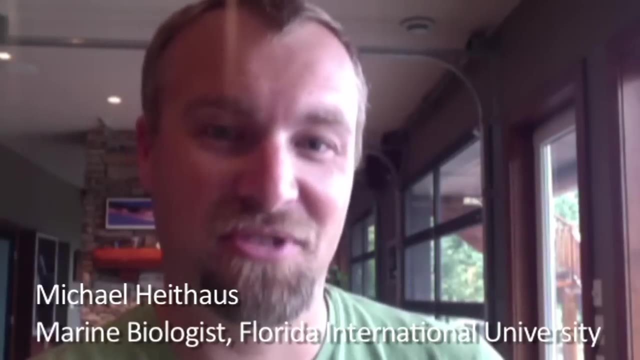 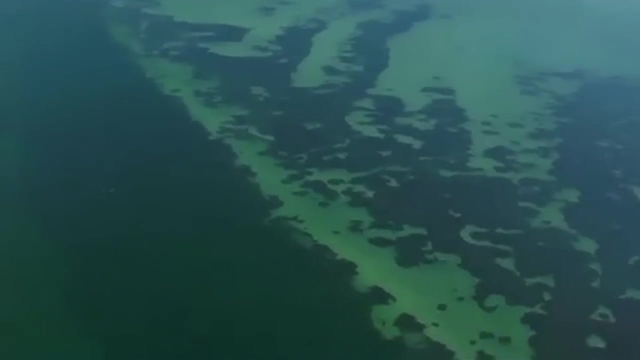 One of the things that we need to know more kind of generally is which sharks are the most important and when are they the most important in ecosystems. So the Shark Bay Ecosystem Research Project started almost 20 years ago, and initially we were interested in dolphins and how they chose where to spend their 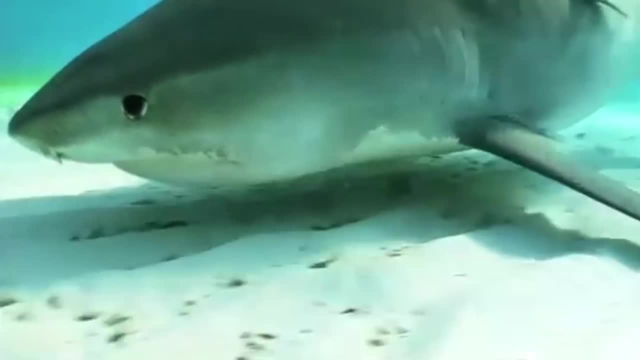 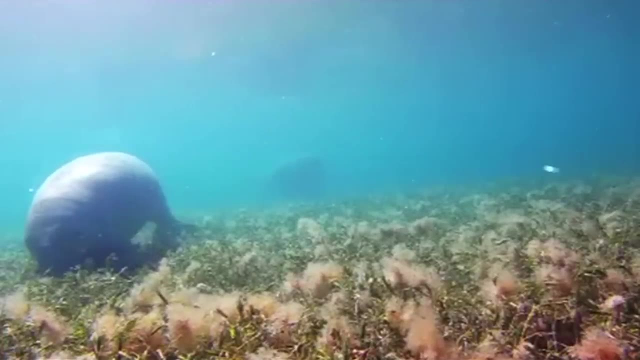 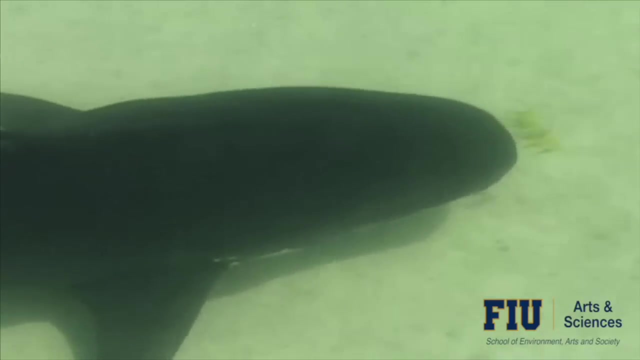 time, but it didn't take long to realize that tiger sharks were a major, important species in this system. So if you want to know how important a top predator is in an ecosystem, that means you have to study pretty much the whole thing. So that means not just the things that tiger sharks eat, like dolphins and dugongs, and 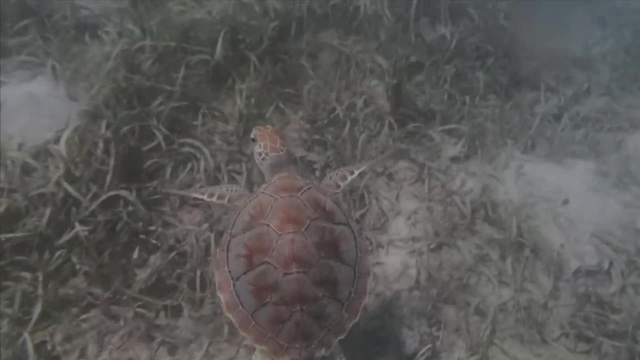 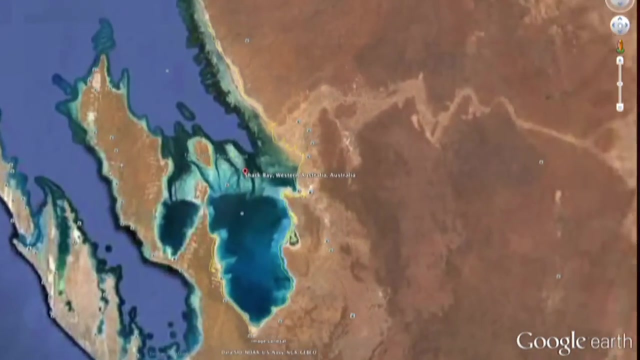 sea turtles, but then the things they eat, the fish and the seagrass. The Shark Bay Ecosystem Research Project takes place in Western Australia about halfway up the coast. We really had an unprecedented opportunity to get to know the shark. We had the opportunity to get to know the 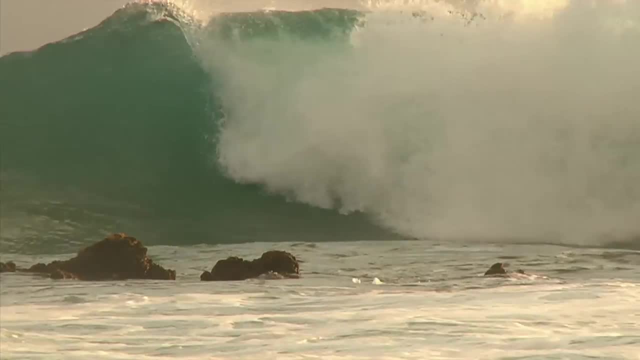 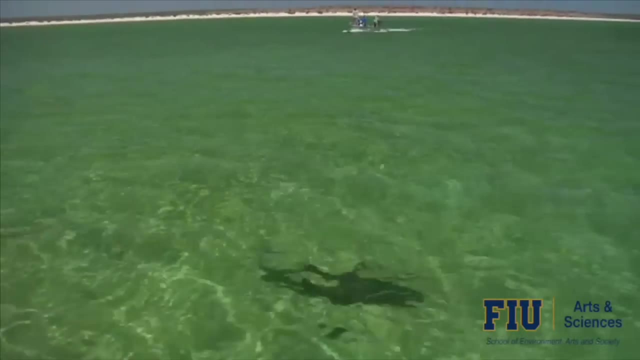 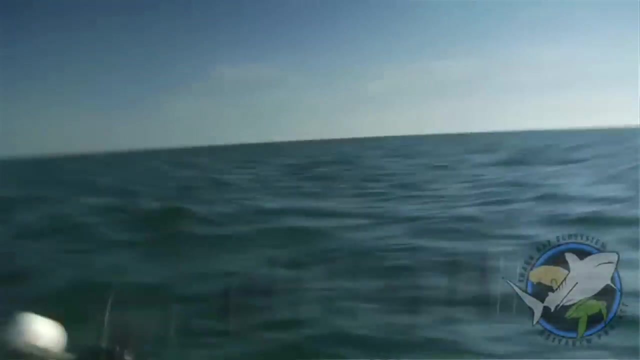 shark. We had to go to a place where the oceans look like they used to hundreds or thousands of years ago, with huge populations of sharks, undisturbed seagrass beds. So the first step in our investigation is to figure out when the sharks are around and how many are there, And we do that by putting out lines. so 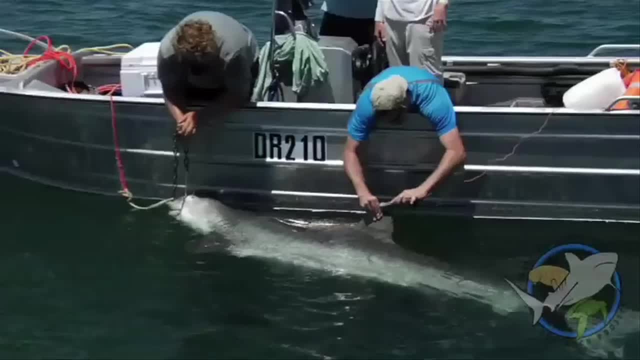 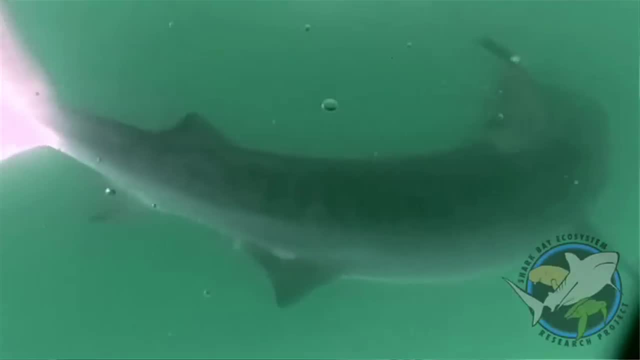 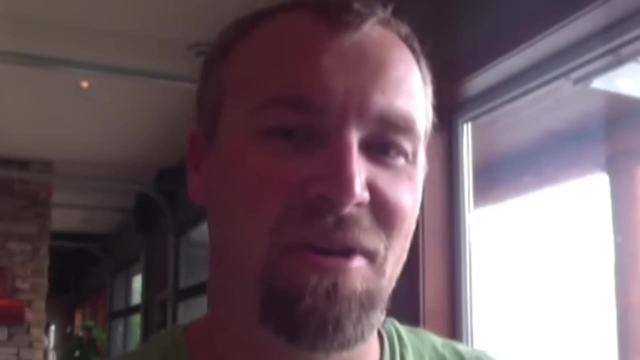 we can catch the sharks, tag them, measure them and then release them. We can then use tracking devices and video cameras that we deploy on the sharks to figure out what habitats they like to spend their time in and where they're hunting. Then we can use data. we 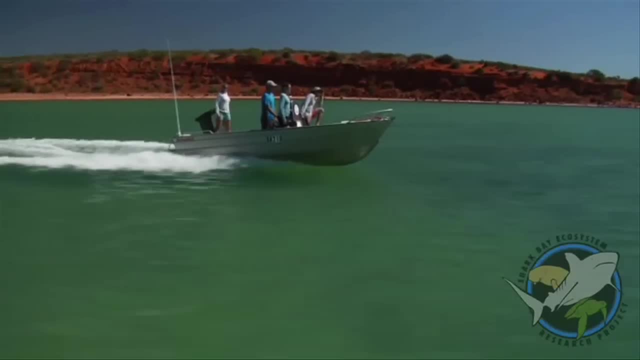 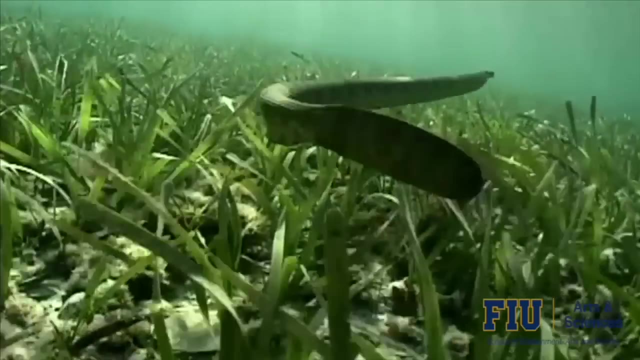 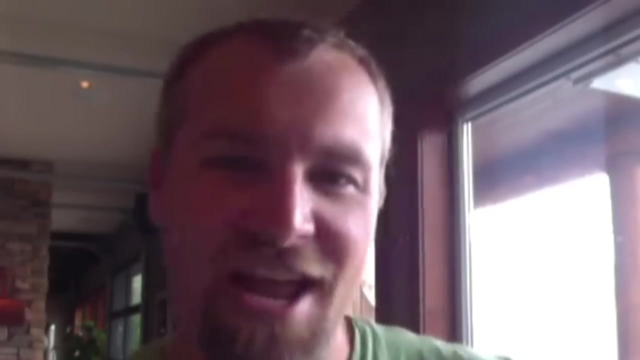 get from driving along shallow and deep habitats. We count all the air-breathing species like sea turtles, sea cows, sea snakes and dolphins, So we know how those animals respond to the presence of sharks. The next step is to figure out how that change in the behavior of those animals. 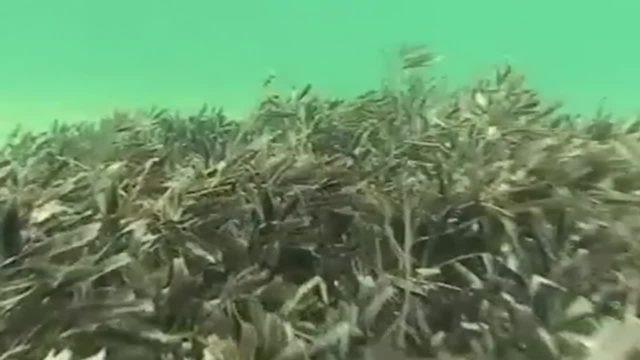 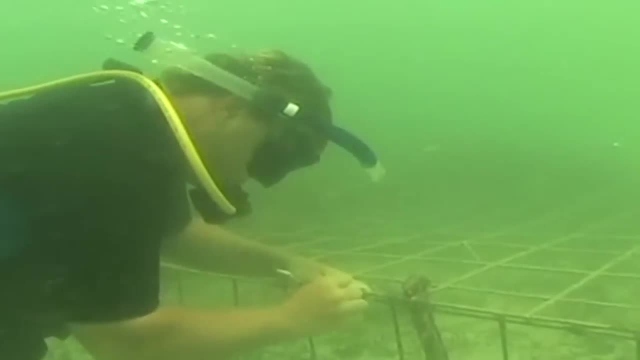 in response to the sharks, affects the seagrass itself. So we build these big cages that are about three meters by three meters. They keep things like dugongs and sea turtles from feeding on the seagrass, And we put those cages in the 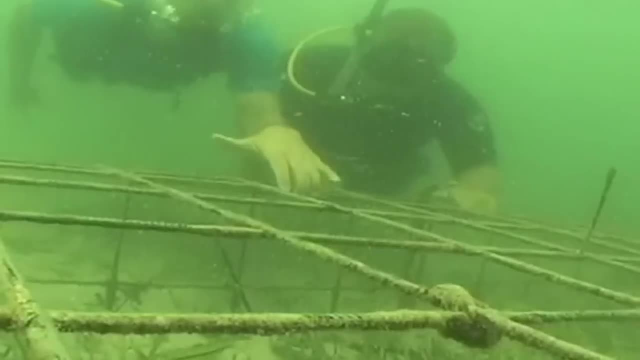 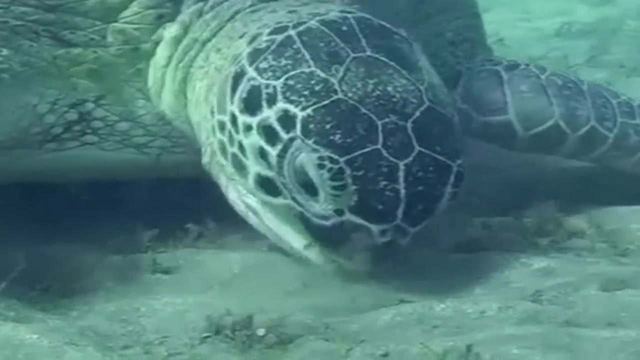 areas that are safe and the areas that are dangerous, to see how much effect they're having. What we found is that in areas where the tiger sharks are really dangerous to these big grazers, it doesn't matter if you put a cage out the